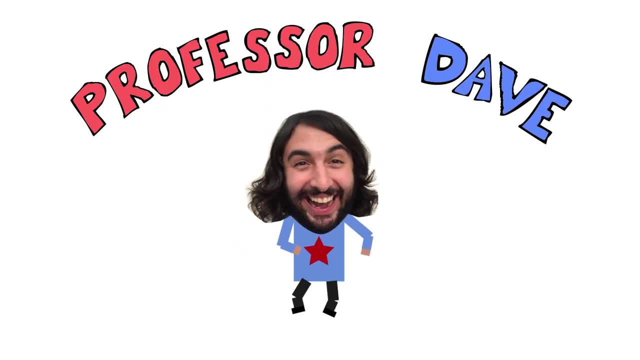 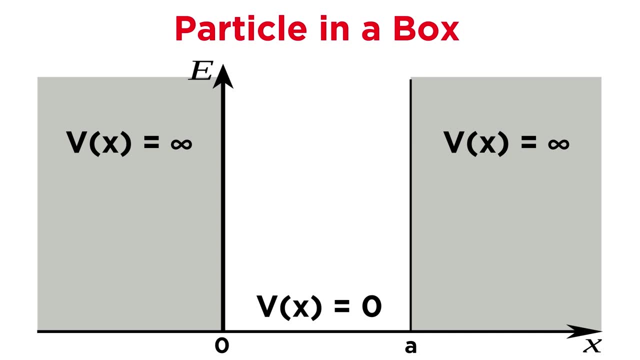 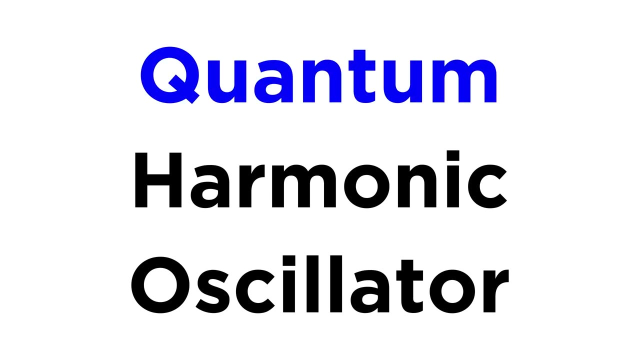 At this point, we have already solved two quantum problems, that of the particle in a box and the quantum barrier potential. Now let's tackle another, which is called the quantum harmonic oscillator. If this term sounds confusing, don't worry. Before we dive into all the math, 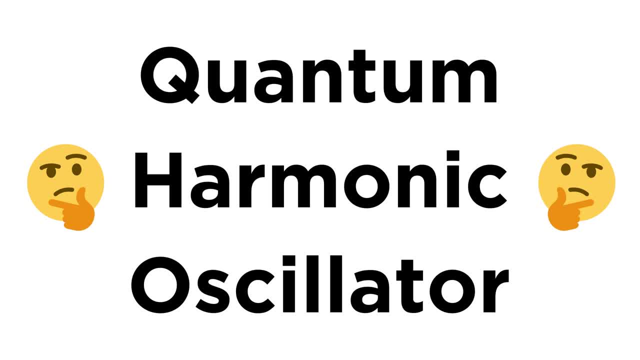 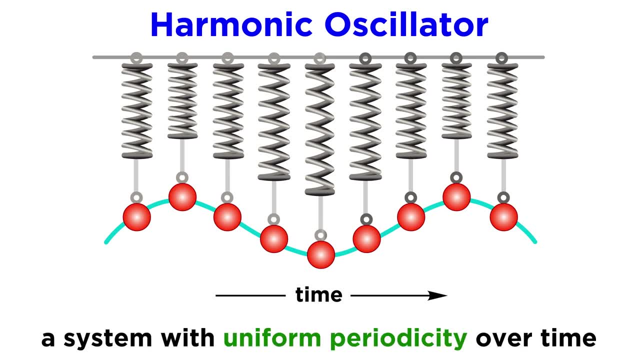 let's just go over a few general concepts for context. First, we must understand that a harmonic oscillator model describes a system with uniform periodicity over time. This is usually referring to a simple sinusoidal wave, which indeed has a reliable periodicity, as opposed to systems that 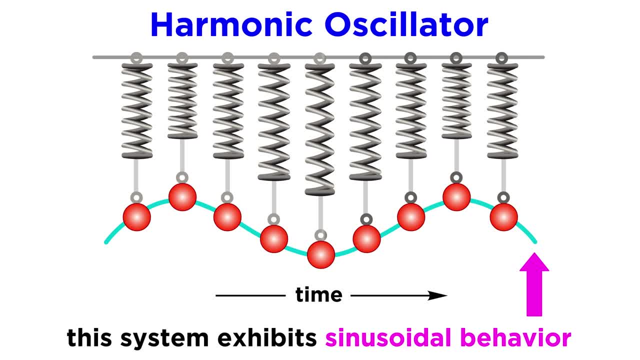 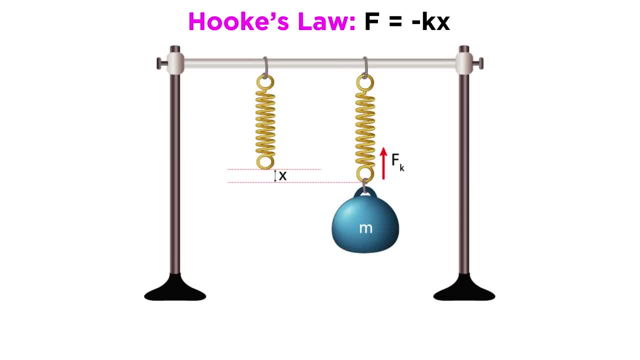 follow more complicated patterns over time which generally would not be referred to as harmonic oscillators. If we can recall our study of Hooke's law and simple harmonic motion, from the classical physics series we can see an example of this type of behavior. This law describes the dynamics of an object with mass m attached to a spring. 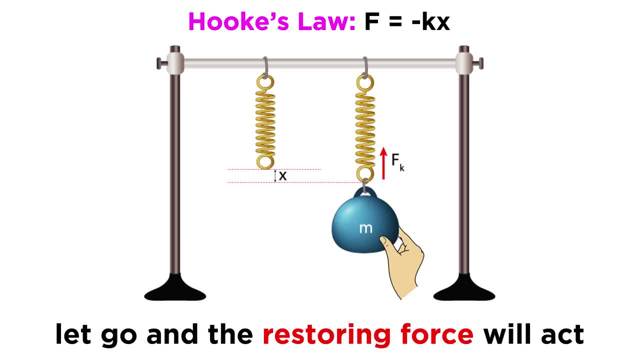 with the spring constant k And specifically, the law tells us that if a particle with mass m is subjected to a restoring force, such as if it is held by a spring, then the mathematical expression for this restoring force is: f equals negative k. 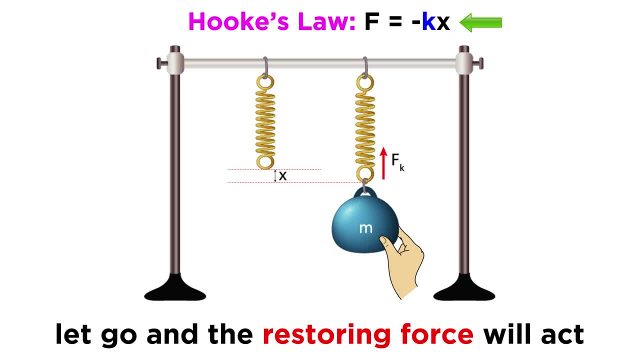 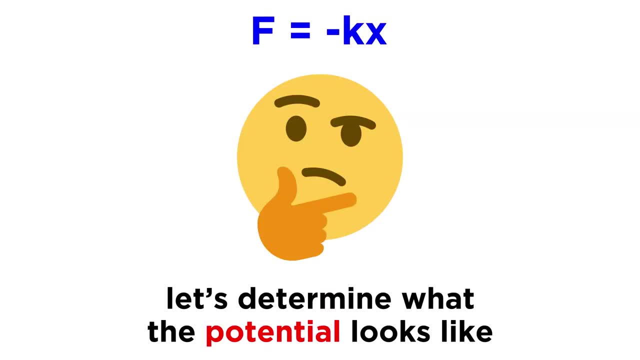 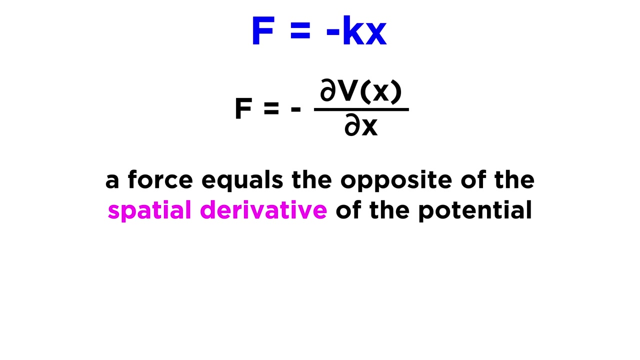 From this expression, we can determine what the potential looks like. To do this, we can use a known relationship between a force and a potential that we learned earlier in the series. This relationship states that a force equals the opposite of the spatial derivative of the potential. What this means is that if we know the mathematical 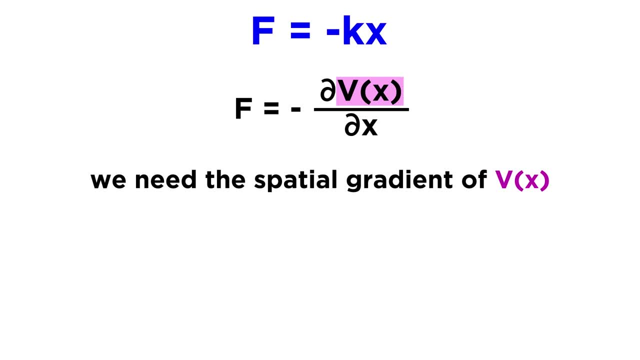 shape of a potential V of X in the scalar form, meaning not as a vector, then we can find the mathematical shape of the force that results from it as the spatial gradient of V of X. That will look like this: To clarify: by spatial gradient we mean a derivative with respect to spatial coordinates. 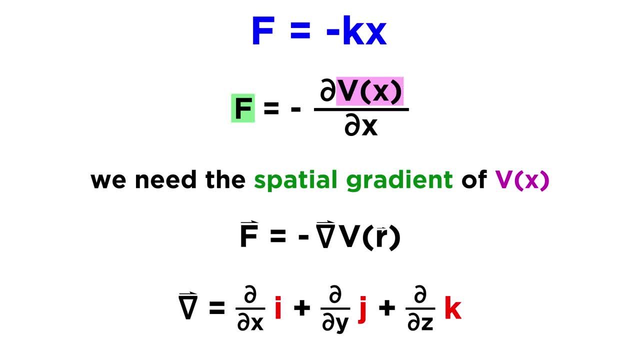 If we think of a three-dimensional system defined by vectors in this form, then we need to take the partial derivatives with respect to the three spatial directions. The negative sign is there because force equals the opposite of the gradient of a potential. It's like 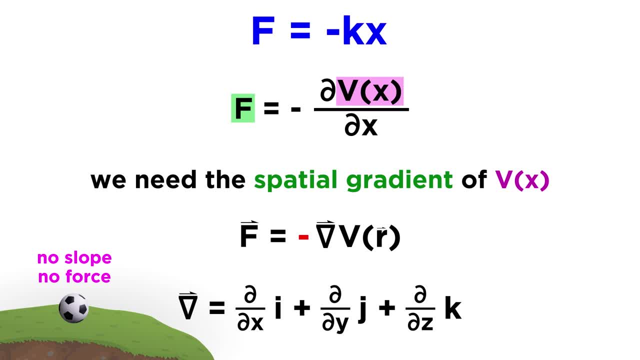 with a ball rolling up a hill. If the ball were in a flat region, the gradient or slope would be zero, and thus there is no force. But going up the slope, the potential energy increases and the ball will feel a force in the opposite direction. down the slope. 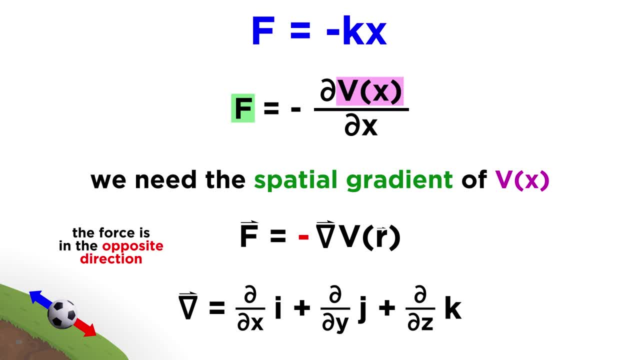 Without the negative sign. it's as though the force would cause the ball to accelerate up the hill and thus travel indefinitely to regions with higher energy levels. So if we think of a three-dimensional system, then we can see that the force will be greater. 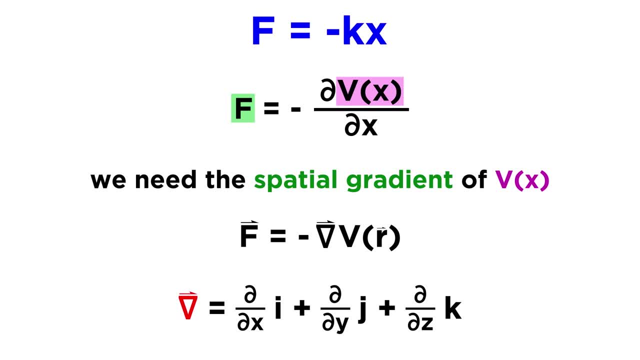 than the gradient or slope, and thus the force will be greater than the gradient. Now we know that the gradient represented by this symbol is equal to the sum of these partial differentials, But if we are dealing with a one-dimensional problem, as we are, 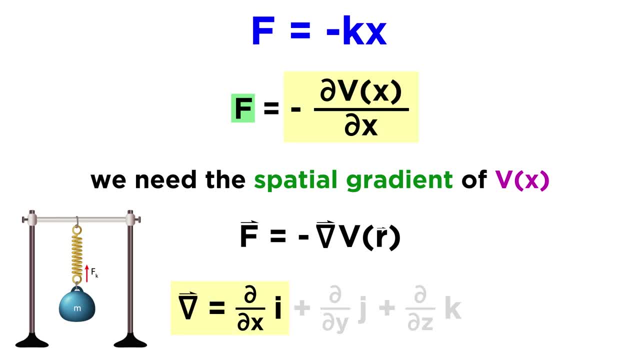 here we can just use ddx. So, applied to the potential, that will look like this: where F equals the negative partial derivative of V of X with respect to X, Intuitively this tells us that a force will be larger where the gradient or. 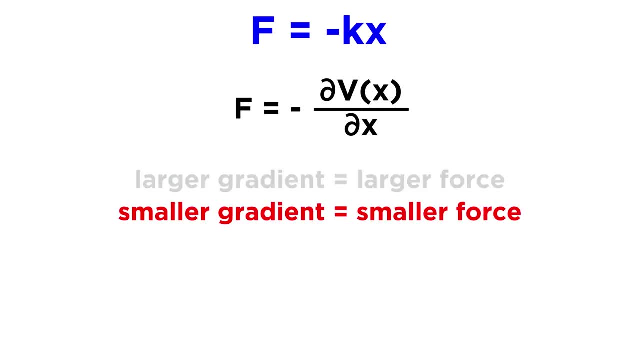 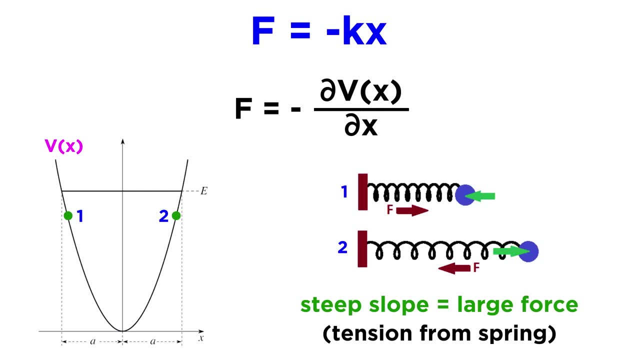 essentially the slope of the potential is larger, and where the gradient is smaller, the force will be smaller. So a flat potential would mean zero force, And a large gradient or steep slope will mean a large force. From here we can substitute Hooke's Law in place of F, so F becomes negative, KX, Let's. 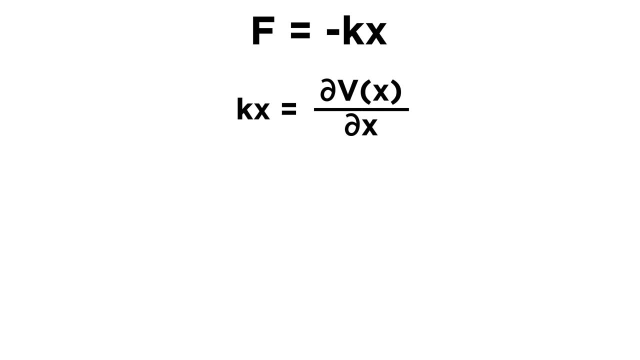 now multiply both sides by negative one to get both sides positive, and then multiply by dx, so that we have KX. dx equals dV of X. Now let's integrate both sides. Don't get tripped up by dV of X. this is not really. 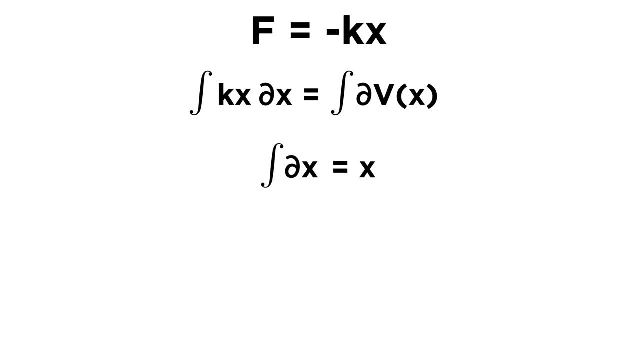 any different than dx, and we know that integrating dx gives us X. so the integral of dV of X will be V of X. Then integrating KX- dx will give us one half KX squared. Now this happens to be the expression for a classical harmonic oscillator: V of X equals one half KX squared. This expression, 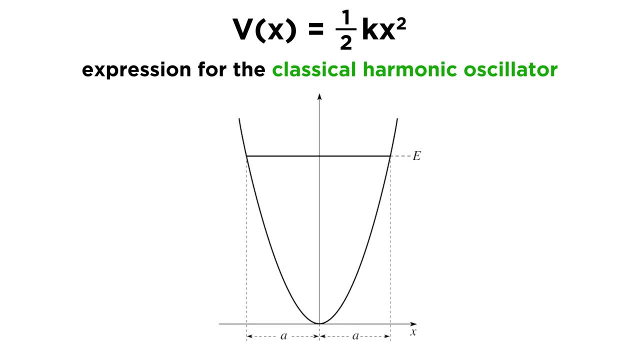 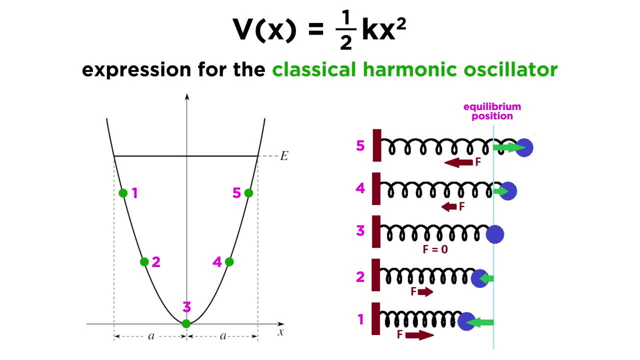 will be very important moving forward, since it describes the energy landscape that a particle encounters in a harmonic potential. What this means is that the expression shows how the potential energy changes with respect to position. As the particle moves in any direction, it will encounter an energy barrier, so to speak, that grows quadratically with respect to X. 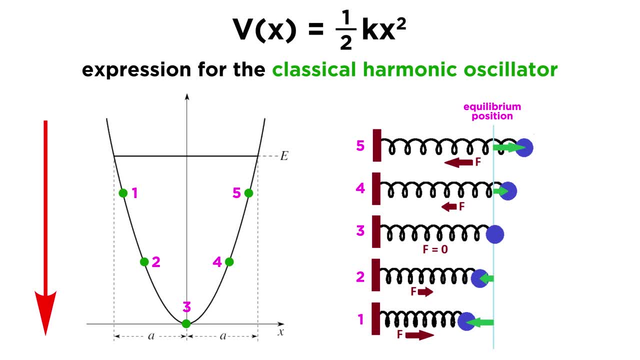 Since the potential energy changes with respect to position, it will encounter an energy barrier, so to speak, that grows quadratically with respect to X. Since we know that any system tends to move towards its lowest energy state, low energy particles will tend to remain at the region with minimum potential energy, which, for one 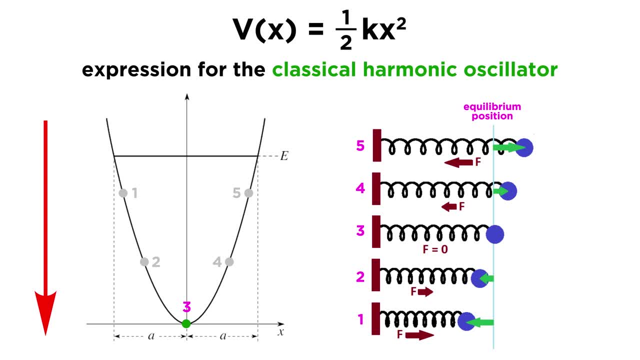 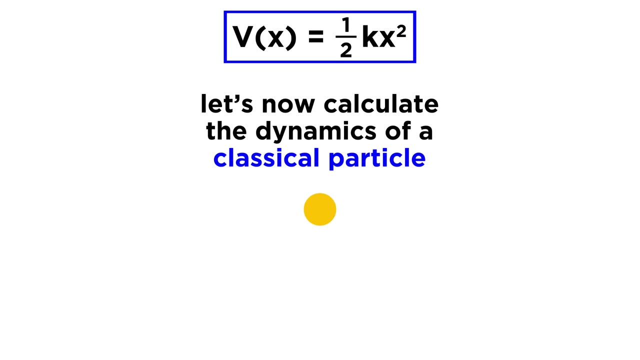 half. KX squared is close to X equals zero. This is essentially like saying that a ball on a spring will tend to remain at its equilibrium point, the point with the lowest potential energy. Now, having defined the mathematical form of the harmonic potential, we are ready to calculate. 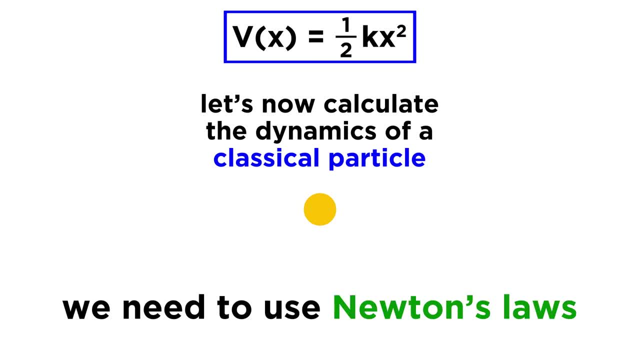 the physical dynamics of a classical particle. To do this, we will use Newton's equations, which we are familiar with from the classical physics playlist. Solving the newtonian dynamics of this particle means finding how the particle's position changes over time when it experiences. 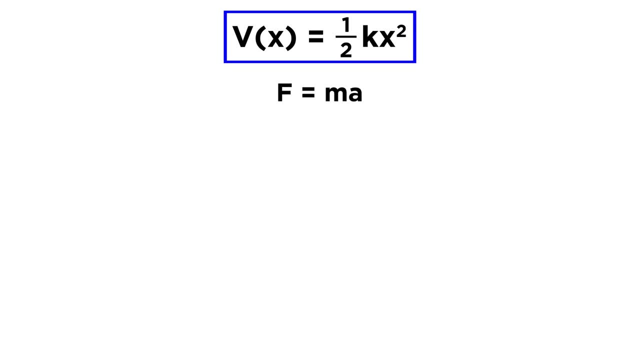 the force that stems from the spatial derivative of the harmonic potential. So let's go ahead and use the equation F equals ma. This equation tells us that the force applied to a particle times the resulting acceleration, and we can express acceleration as the second derivative. 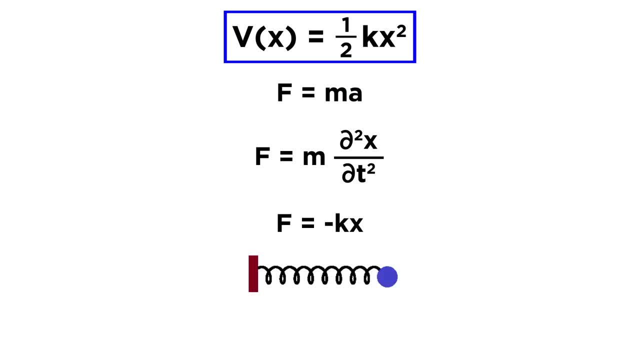 of x with respect to time. Once again, we also know that f equals negative kx, which is the force applied to the particle by the spring. So let's substitute this expression for f in our equation, and now we have this. This is a second-order differential equation which we can 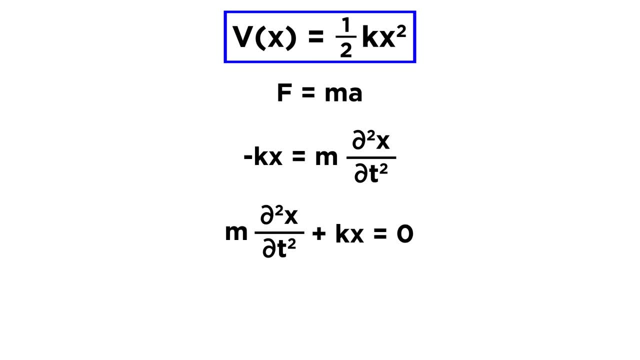 now solve. First, we have to rearrange things a bit. Let's get both of these terms on the same side, with their sum now equal to zero, and then let's divide through by m. To simplify a bit further, let's define a constant beta which is equal to root k over m. That means we can place 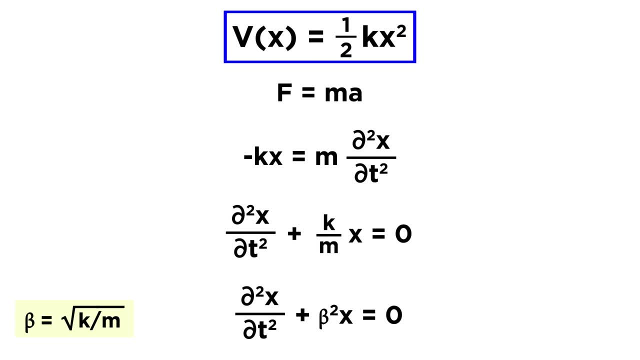 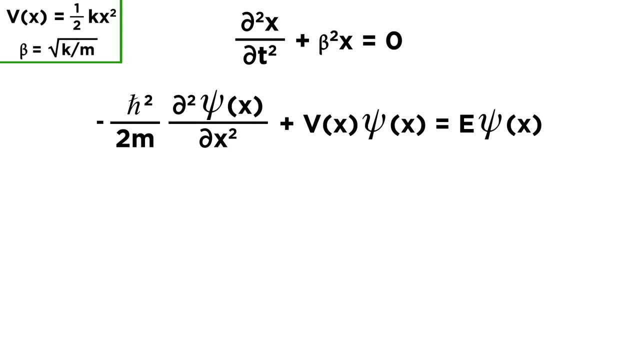 beta squared right here. Now we are ready to solve. To speed up the solution of this second-order differential equation, let's compare this equation with the Schrodinger equation. Even though they represent completely different physical realities, we may recognize that this equation looks like the Schrodinger equation, with a potential that. 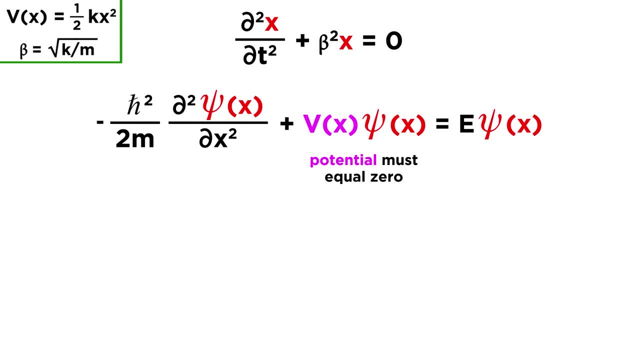 equals zero and where psi of x is substituted with simply x. To make things more clear, let's set v of x equal to zero, so we can get rid of this term and then move the e term to the left side. To go even further, in previous tutorials we have rearranged this to look more. 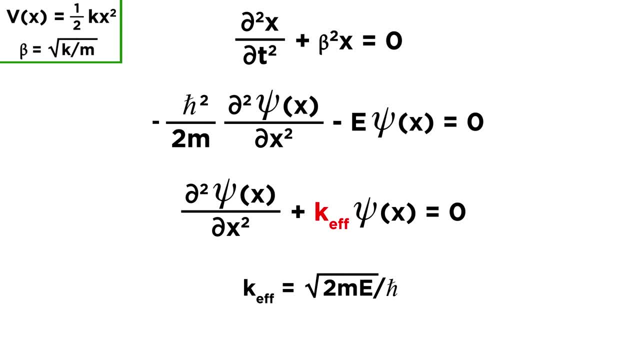 like this, with the constants contained in this other constant k, which equals root two m e over h bar, And here we've also multiplied both sides by negative one to get everything positive. And now in this form we can really see the similarity between our original equation. 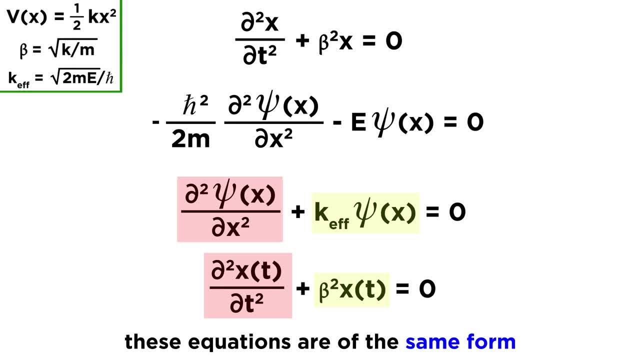 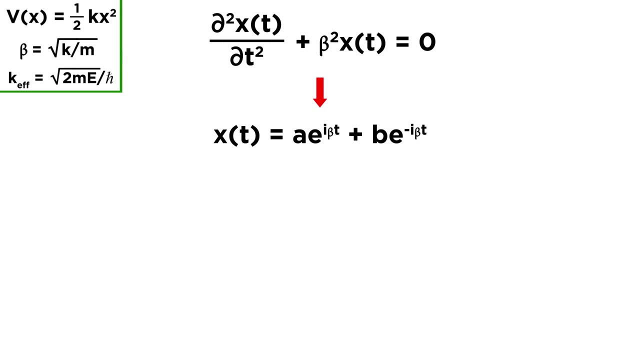 and the Schrodinger equation, We simply have x of t instead of psi of x. Making this comparison is useful because we have already solved this equation in earlier tutorials, so we know the solution for x will be a linear combination of complex exponentials, as we see here And again, like with previous tutorials, we can solve this equation. 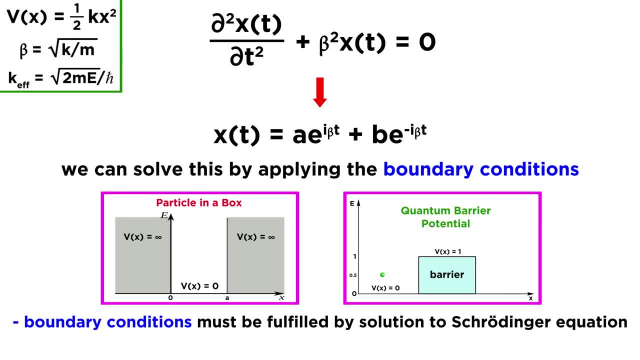 simply by applying the appropriate boundary conditions. Remember that with the particle in a box and with the quantum barrier potential, we had to make sure that the boundary conditions are fulfilled by the solution for the Schrodinger equation to yield continuous functions and either zero or non-zero values, as deemed necessary by the nature of the problem in question. 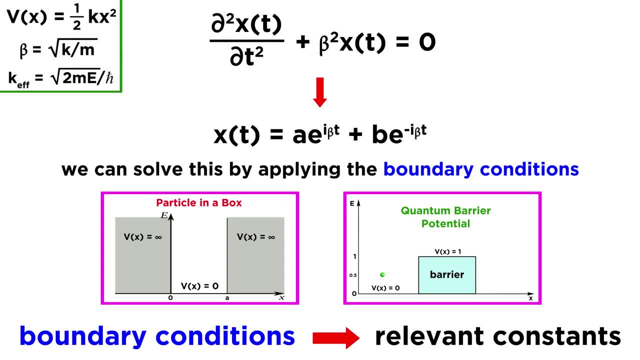 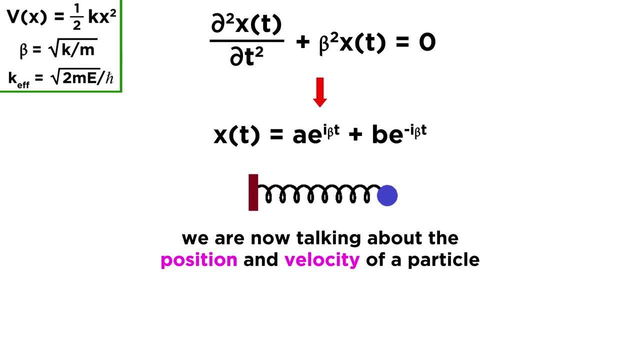 In these cases, we applied boundary conditions for the wavefunction in different regions and thereby found the constants that were multiplying the complex or real exponential terms. In this situation, instead of a wavefunction in different regions, we are trying to find what kind of shape, so to speak, the position and velocity of a particle must have, as dictated. 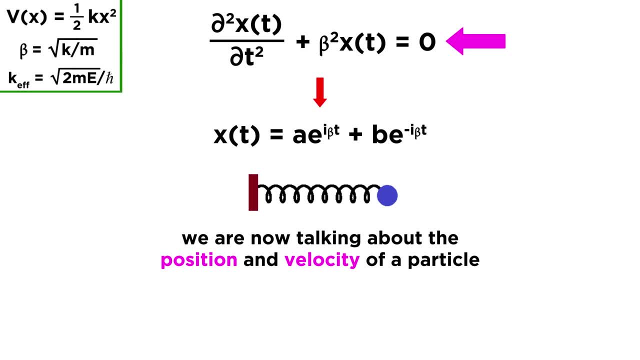 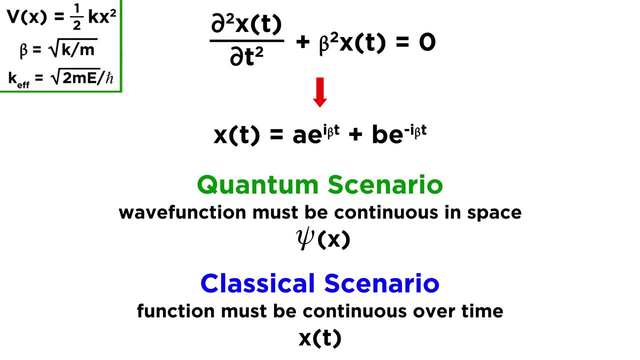 by Newton's equations, more specifically this partial differential equation. So the main difference is that for any quantum, quantum situation we need the wavefunction to be continuous in space, as psi of x depends on x, whereas with the classical particle we need continuity over time, as x of t depends. 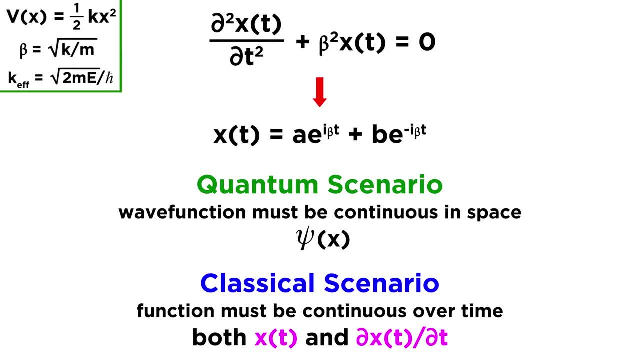 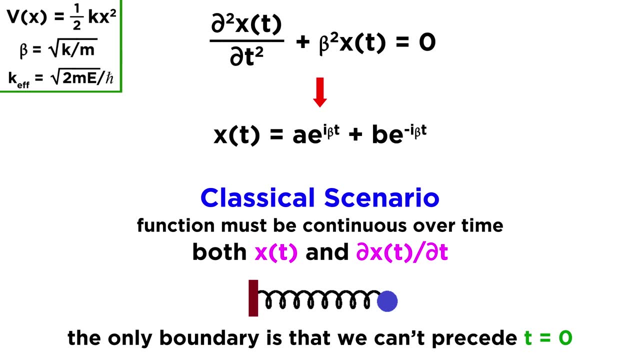 on t And recall that the continuity condition requires that both x of t and its derivative dx of t over dt must be continuous. In addition, the interesting thing here is that, unlike what we are used to with boundaries for x, there are no time boundaries except that. 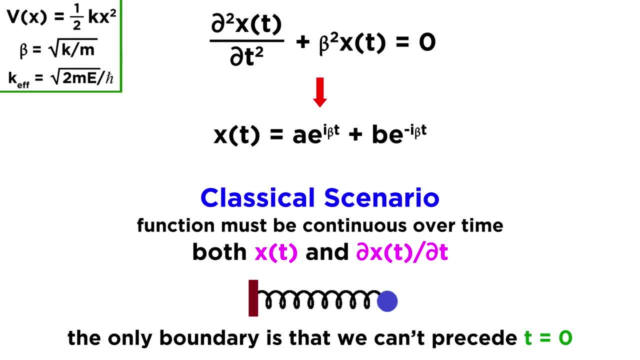 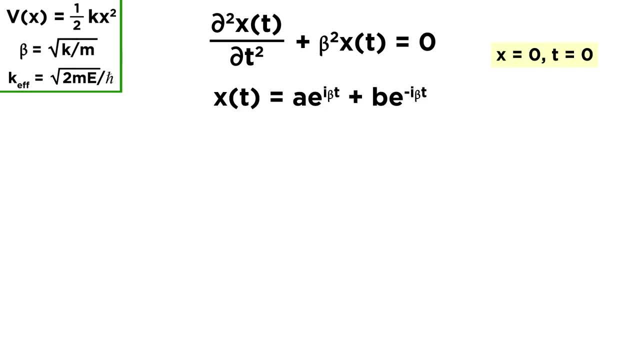 we cannot precede the time t equals zero. so for this reason, we will solve the time continuity equations only at t equals zero. Now, with all of that understood, let's say that our particle is at x equals zero, at time t equals zero and that its velocity. 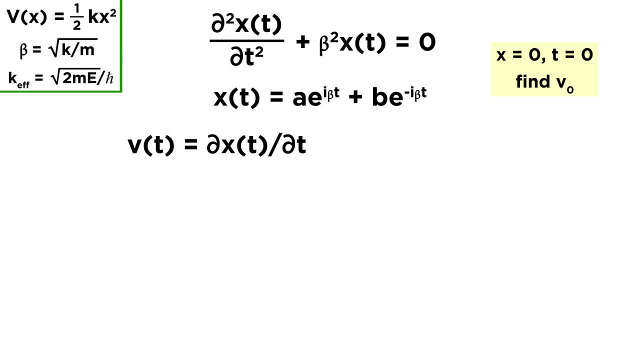 given by v equals the partial derivative of x with respect to time is some constant velocity, v naught. Let's apply these boundary conditions to the equation, starting with velocity. So v zero will be equal to dx of t over dt evaluated at zero, which means we have to take the derivative. 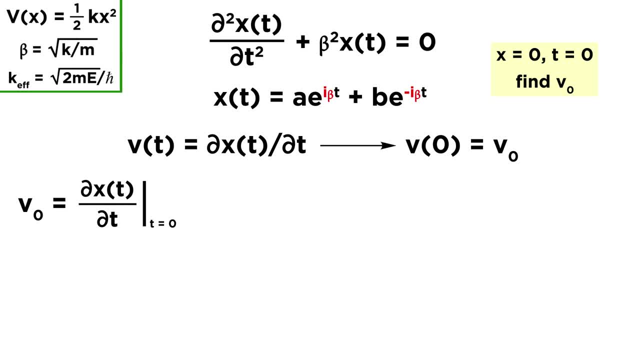 of this expression with respect to t. This just means bringing these constants out front for each term. so we get ia beta e to the i beta t, minus ib beta e to the negative i beta t. Evaluating at t equals zero makes both exponents zero and anything to the zero. power is one. 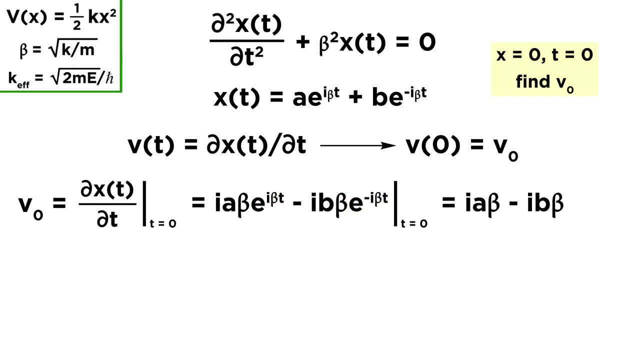 so the e terms essentially just go away, leaving us with ia, beta minus ib, beta Again. we will call this v naught. Then for the second condition, we know that x equals zero at time zero. so x of t becomes x of zero, and we can set that equal to zero. This turns these exponents into zeros. so 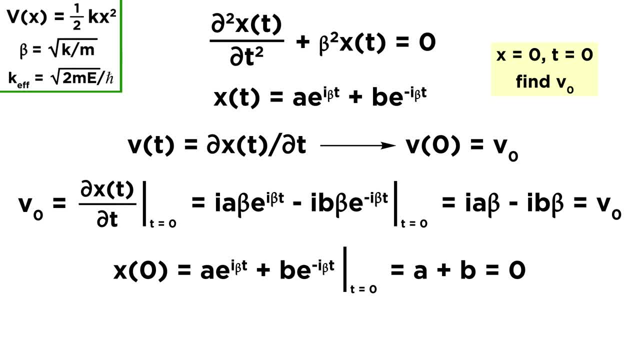 these come equal to one, and we are left with a plus b equals zero. So here is the resulting system of two equations. This is trivial to solve using basic algebra. We can just multiply the second equation by i beta, and then we simply add them together. 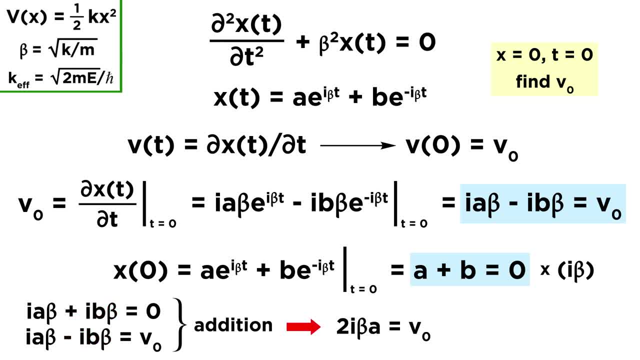 The second terms cancel out and we are left with two. i beta a equals v. naught Rearranging to solve for a. we get this. Let's take this and plug it into the original second equation, which will allow us to then: 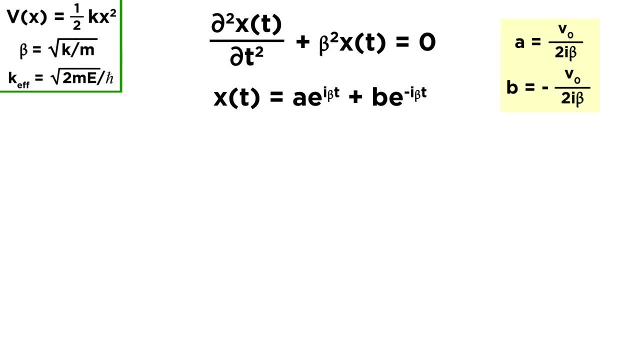 solve for b. With values for a and b, we can now solve for x of t. We just plug these new expressions in for a and b. To simplify, let's factor out this expression, leaving this parenthetical with the exponential terms. 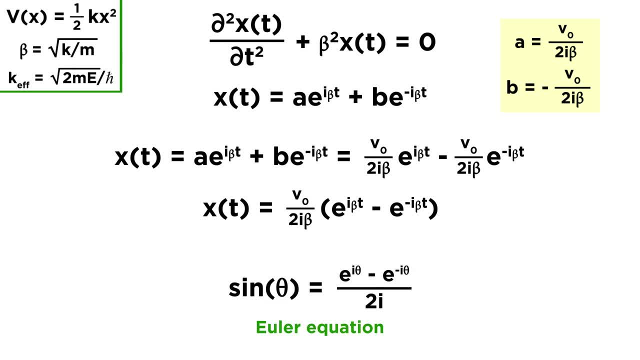 Now we can get clever. We have used this Euler equation a few times by now and we can recognize that it has the same value as the first equation. It's the same form as the equation we currently have. we just have beta t in place of theta. 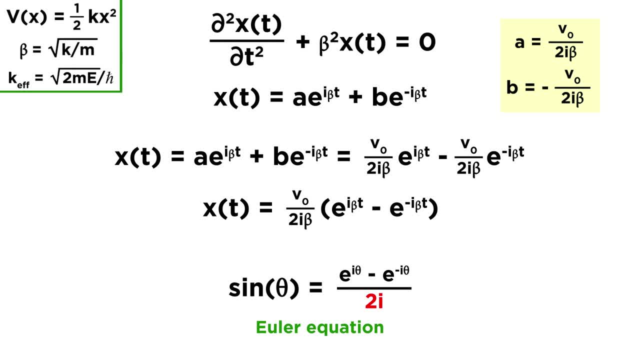 We just need this expression to be over two i in order to make the substitution. so let's multiply by two i over two i. These ones over here cancel out, leaving us with v naught over beta and then the other part we can now write as simply sine of beta t. 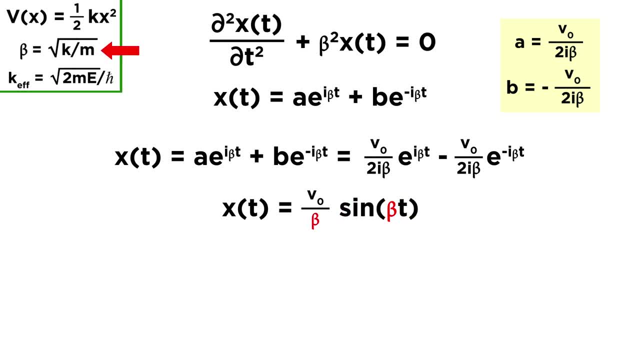 Finally, recall that beta represents root k over m. So let's change the betas back to their original form With beta in the denominator. here we simply invert the expression so we can write root m over k And then root k over m can be written into the sine term. 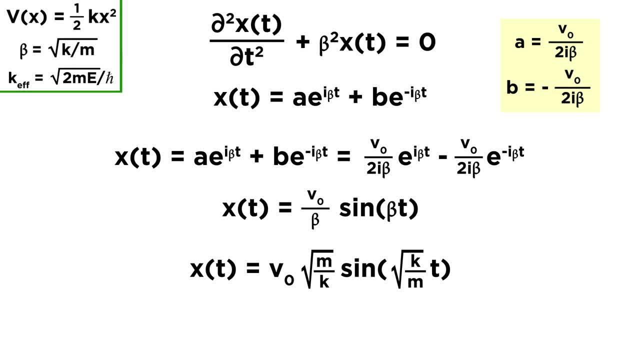 And there we have our expression for x of t. The important thing to understand is that our expression for x of t contains a sine function. That means the particle experiences an oscillatory behavior. The expression for x of t contains a sine function. This is an oscillatory behavior that looks just like a sine wave. 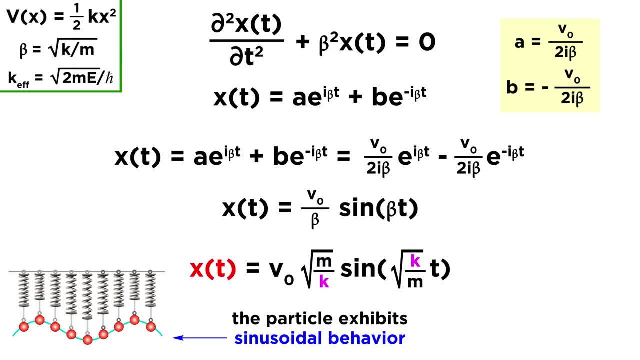 Its position depends on its mass, the spring constant k and the initial velocity v naught. We can define the angular frequency of oscillation omega as being equal to the term within the sine function, or root k over m. This will come into play a bit later. 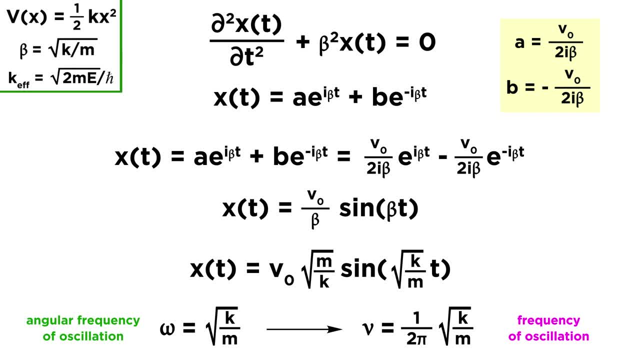 The frequency of oscillation is simply the angular frequency divided by two pi, and this is much more straightforward. It's measured in hertz and just represents the number of oscillations per unit time. Let's pause for a moment here. What we must understand is that, mathematically speaking, the particle can oscillate at any 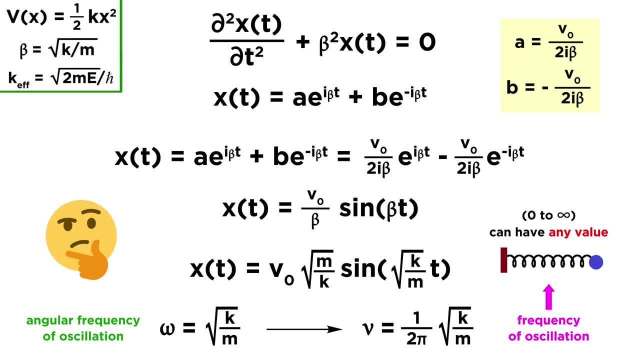 frequency from zero, which means no oscillation at all, or a particle at rest up to any number you can think of. For example, if the mass is 200 grams and k is 0.2 newtons per meter, then the particle 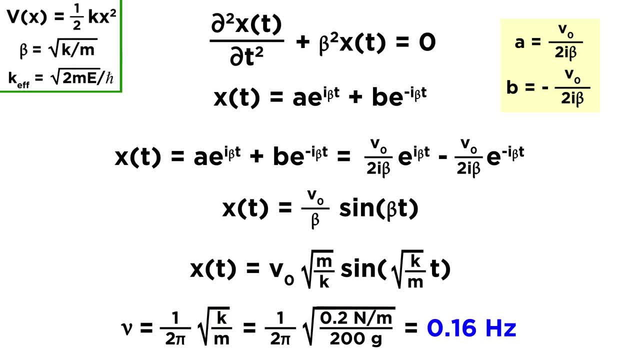 would oscillate at a frequency of 0.1 k. If the mass is 200 grams and k is 0.2 newtons per meter, then the particle would oscillate at a frequency of 0.16 hertz, which is roughly one full oscillation every six seconds. 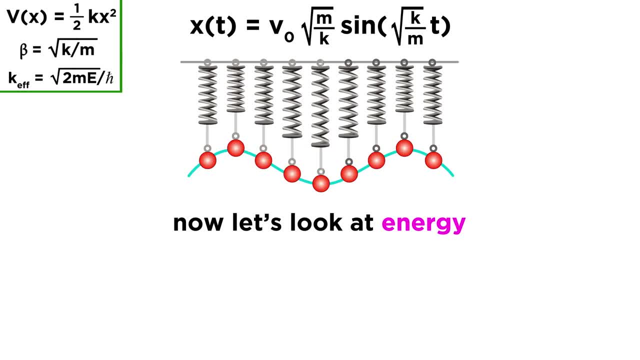 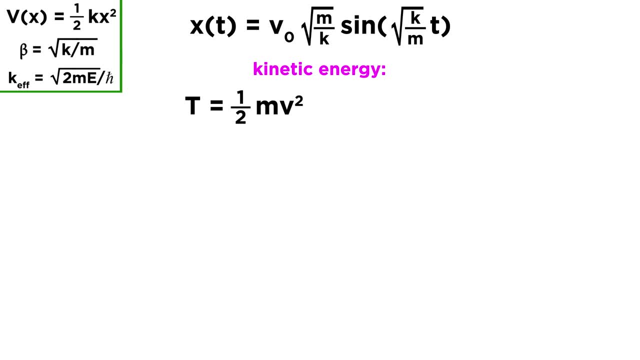 Now let's have a look at the particle's energy as it follows these oscillatory dynamics. The particle's kinetic energy is given by this expression which we are familiar with from classical physics. As we have been doing, let's change velocity to the derivative of position, with respect. 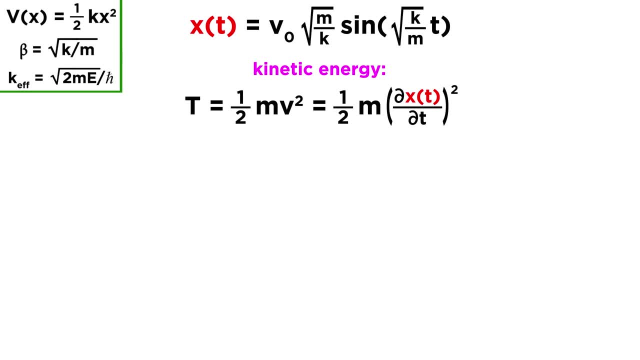 to time. Now, we just solved for x of t, so we should be able to take its derivative. Because we have just solved for x of t, we should be able to take its derivative. Because we have just solved for x of t, we should be able to take its derivative. 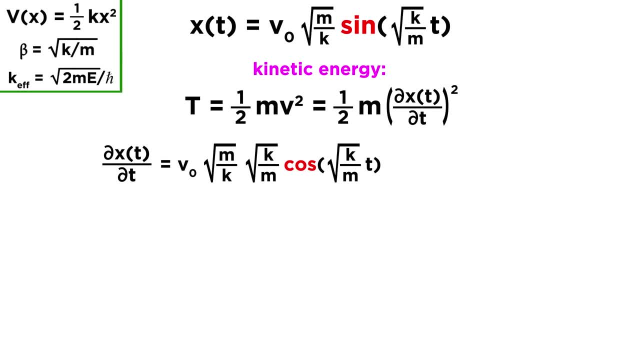 Because it is a sine function and the derivative of sine is cosine. we will get the same expression, but with cosine multiplied by what was inside the sine function because of the chain rule. so root k over m comes out front Conveniently. root m over k times root k over m equals one. so we are left with v-naught. 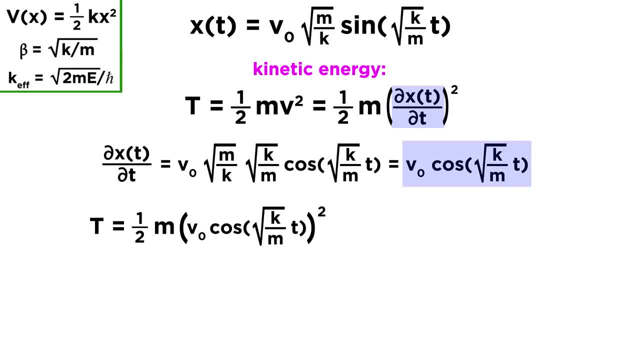 times this cosine term. Now we can go back to our equation for kinetic energy and plug this expression in where we see the derivative. Now this must be squared so that just means we get v-naught squared times a cosine squared term. This is simply the well-known kinetic energy equation. t equals one half m v-naught squared. 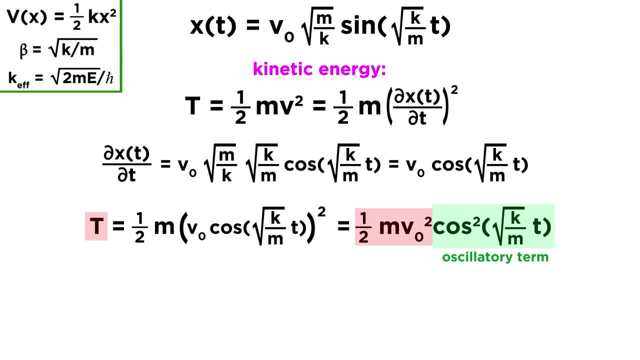 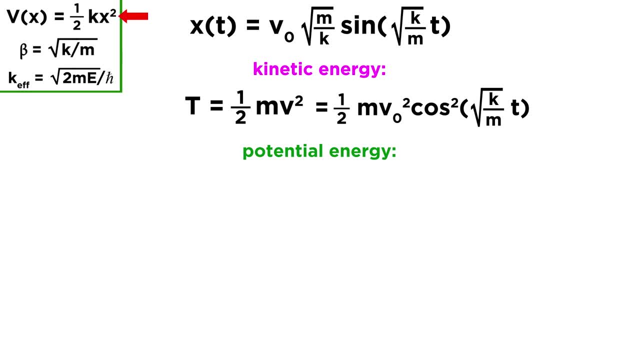 but now with an additional oscillatory cosine. squared term Potential energy is also quite trivial to solve for, since we defined it earlier as follows: v of x equals one half k x squared, or now x of t squared. Let's plug in our expression for x of t and then square it. 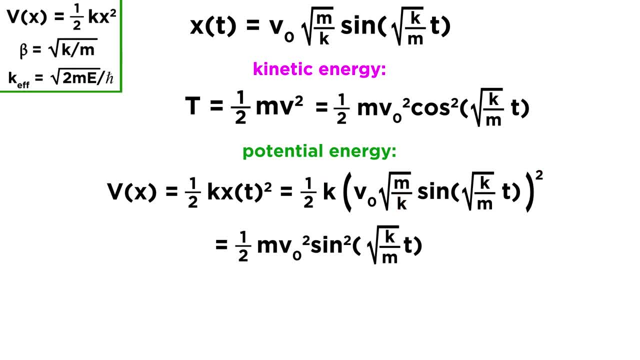 The k's out front will cancel out, and we get this precisely the same expression as for kinetic energy, just with a sine squared function instead of cosine squared. Now, the total energy of the system E will be equal to the kinetic energy, t plus the